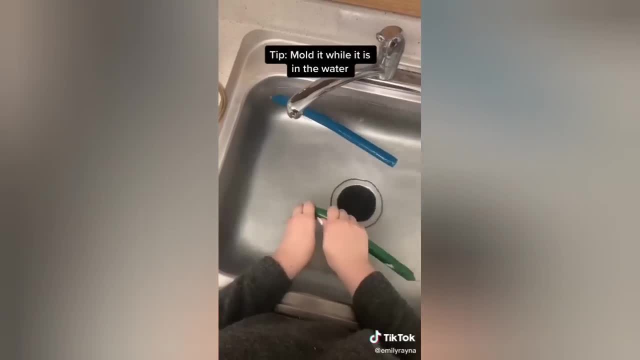 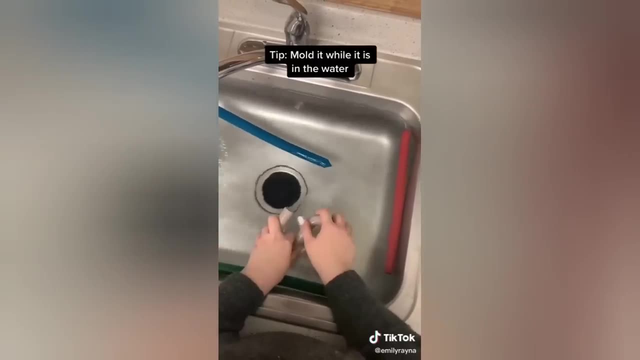 you can see I had some errors at the start, but what I discovered is that if you mold it while it's still in the hot water, it works a whole lot better. There was no cracking at all when it was in the water and I cut the bottom off of some of them to make them stand better and I sandwiched. 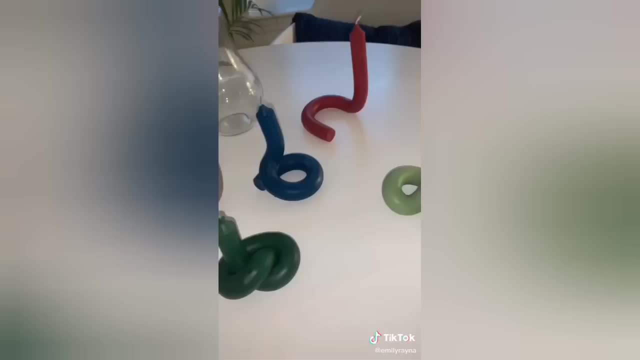 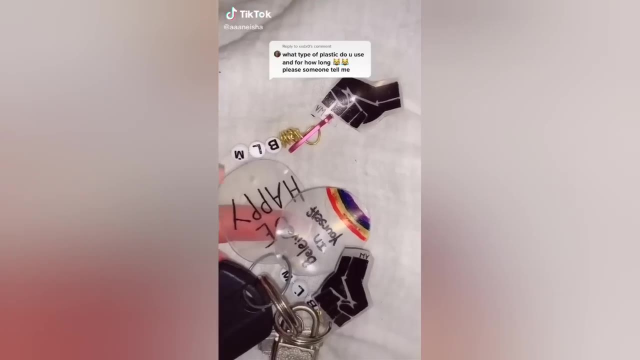 them between things while they dried. and these are the results. I think they're so much fun and I hope this helps you guys. I used number six plastic to make these. You could use shrinky dinks, but I don't know if you can see it. I used number six plastic to make these. You could use. 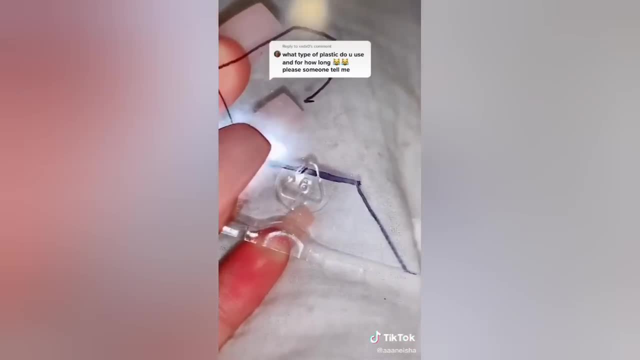 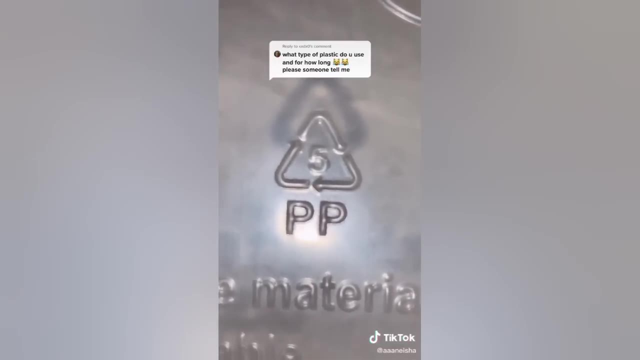 I would recommend using recycled plastic just because it's better for the environment, but it looks like that The number is inside of the triangle thing. If you use anything else, you'll probably set your house on fire. but whatever you're drawing, make sure you do it like a pretty. 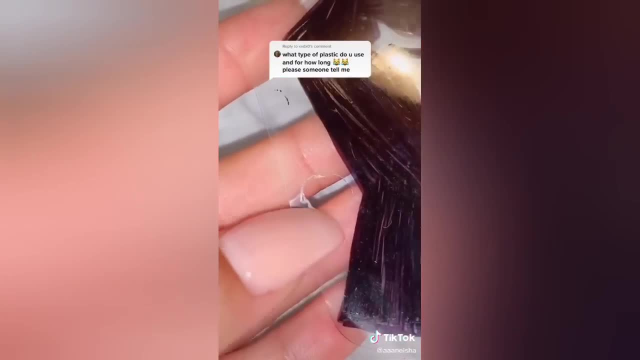 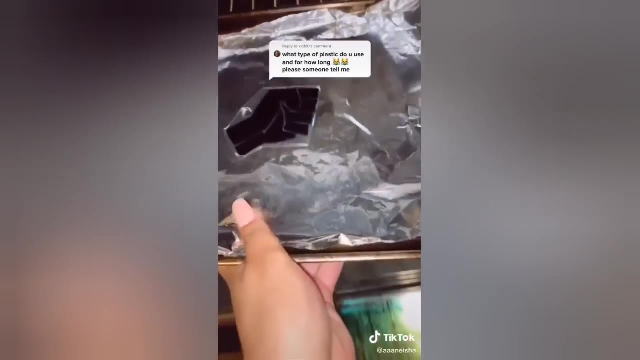 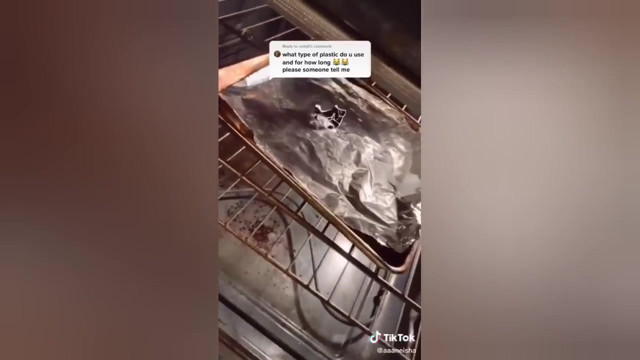 big size because it'll shrink a lot in the oven and punch a good size hole- 350.. Foil line baking pan into an oven. Turn the oven light on so you can see, but it'll burn. I'm going to use a twelve inch baking pan with a bending screw which will sit right here so it stays flat. 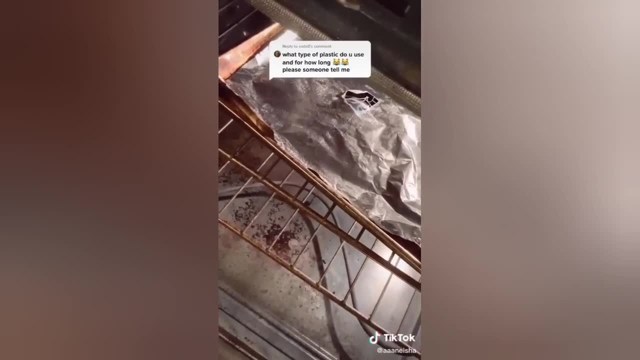 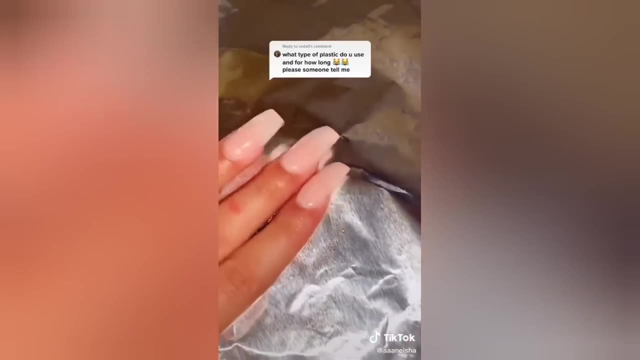 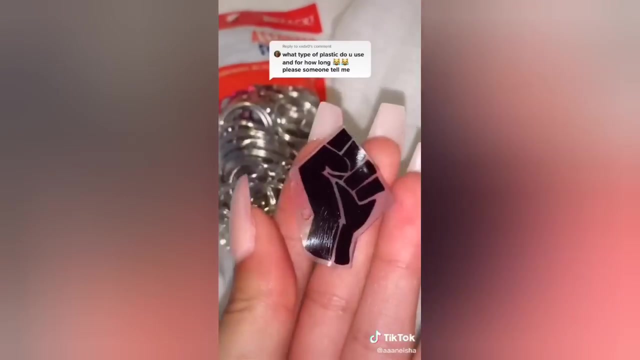 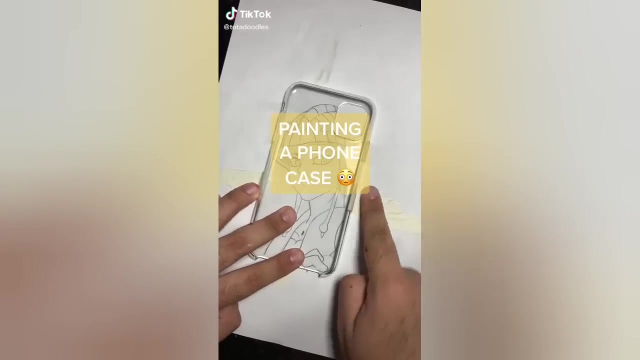 One of my favorite tools is this. Please don't know how to attach it. The coasters suck, actually burn or do anything, and the solution works really well. It's like a creativity package and, through the em, fills you with brushing ever so thoroughly. Try painting deep by fading down, and you could. 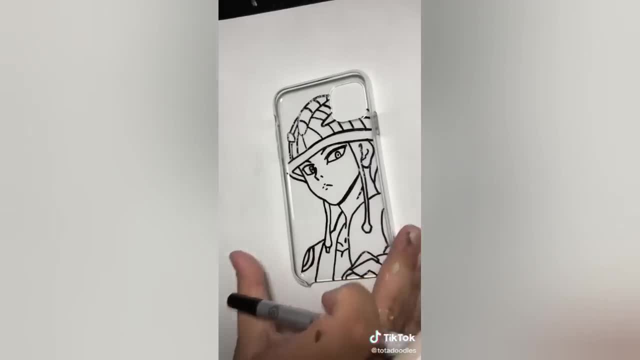 completely curl up like this, Like that, And you kinda just have to sit there and watch it until it and we're going to be painting a phone case for a special order from a client. after i retrieved the proper phone case for them, i started painting and i was very careful about where i was laying paint. 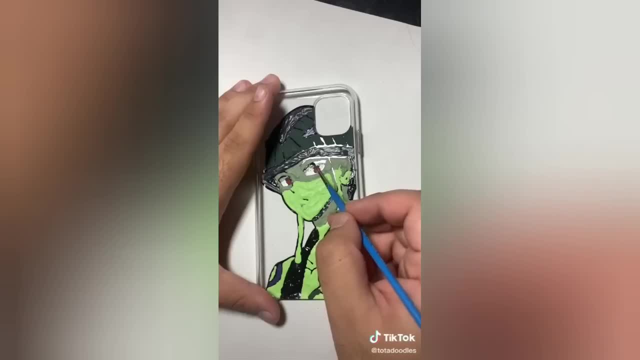 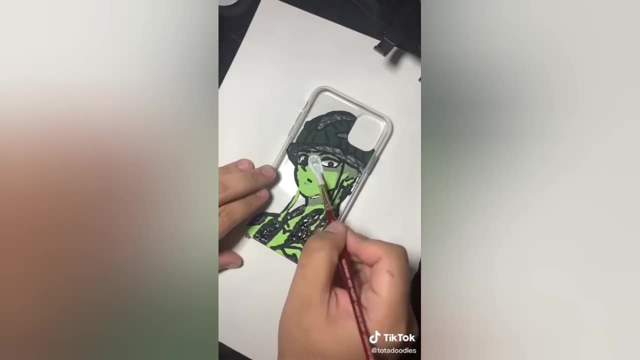 because i didn't want it to seep out of the outline. after that i went and put black paint over the black marker and then after that i put a layer of sealant behind the paint after it dried. after i put the first layer, i've laid down a second layer just to give it that extra protection. 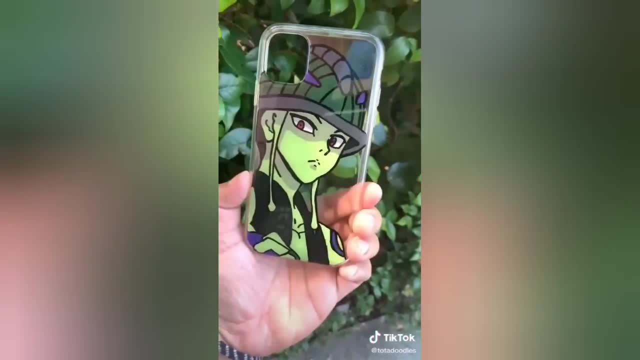 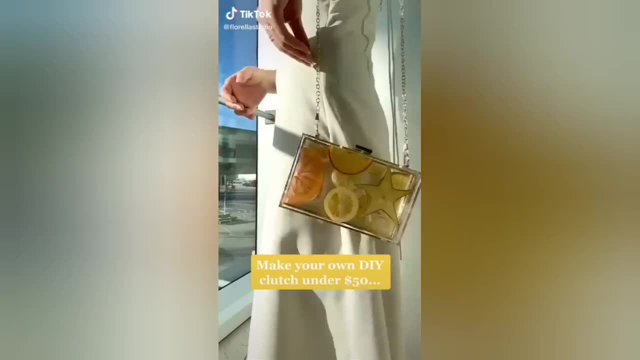 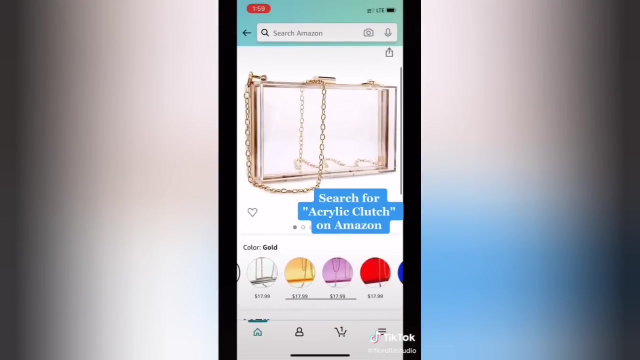 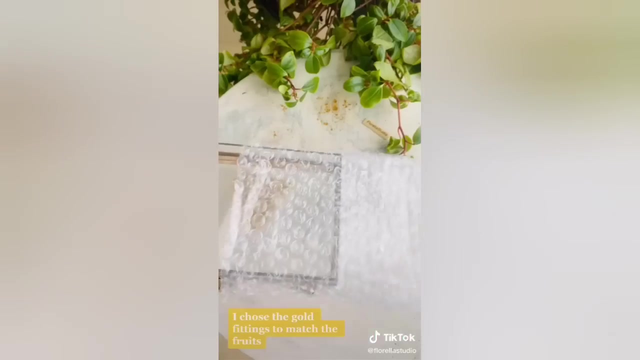 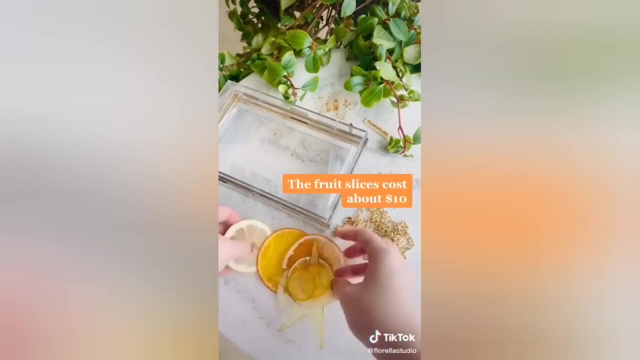 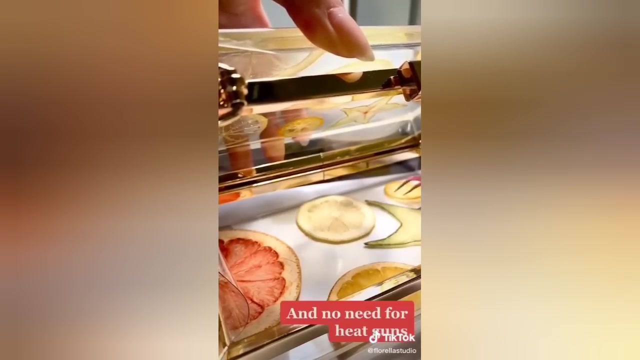 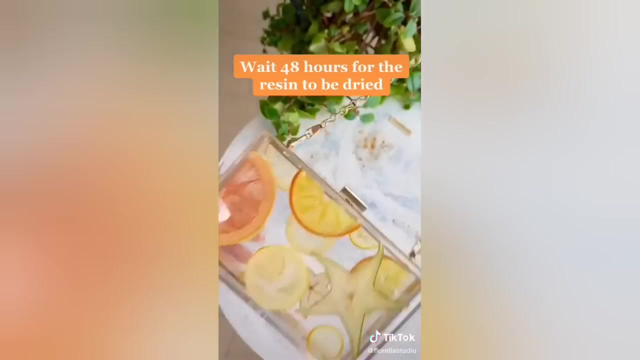 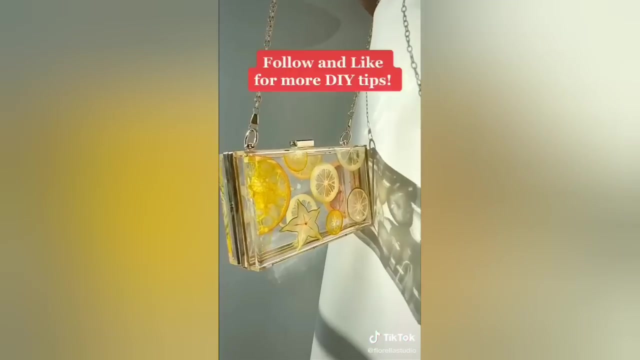 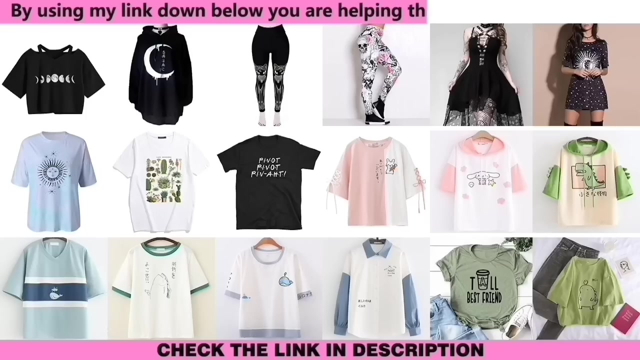 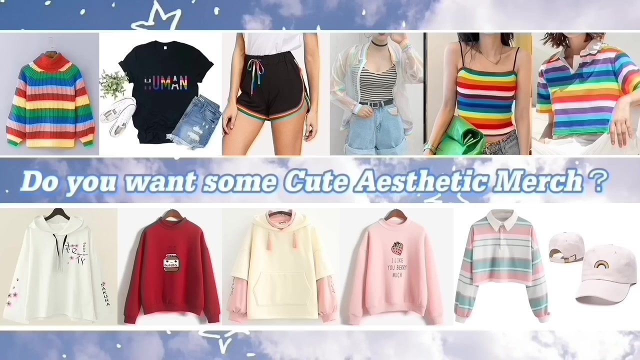 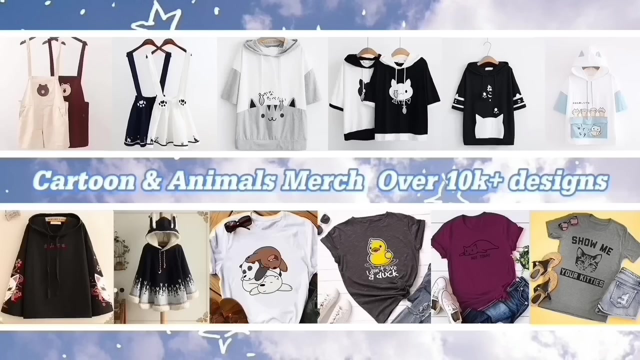 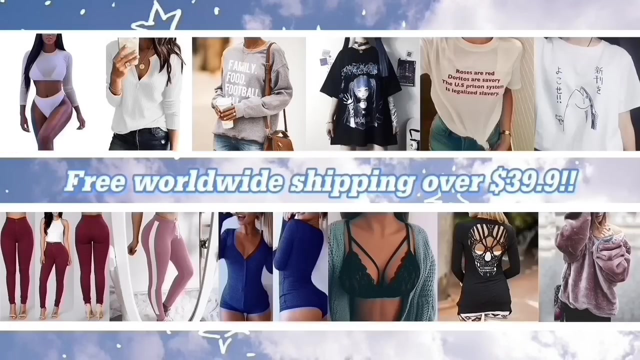 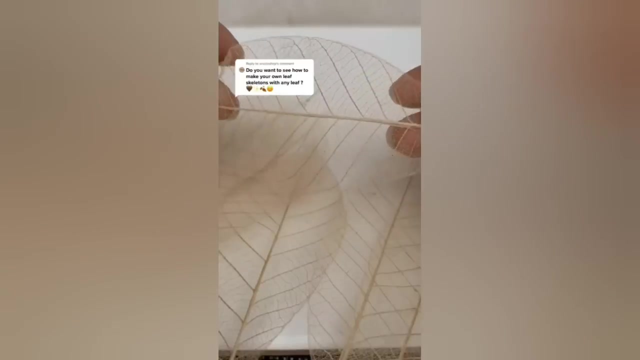 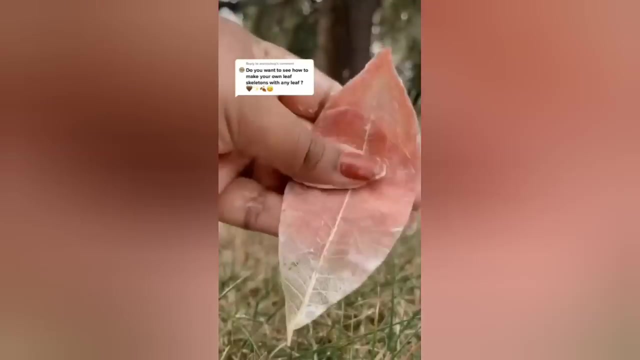 and then in the end it looked like this. it's pretty cool. i like it, so, so. so a ton of requests to make your very own leaf skeleton that we use in our signature leaf soaps. remember, it takes patience and persistence. first step is to choose your leaves. 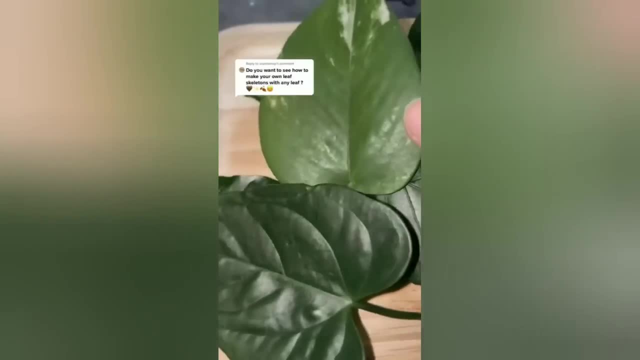 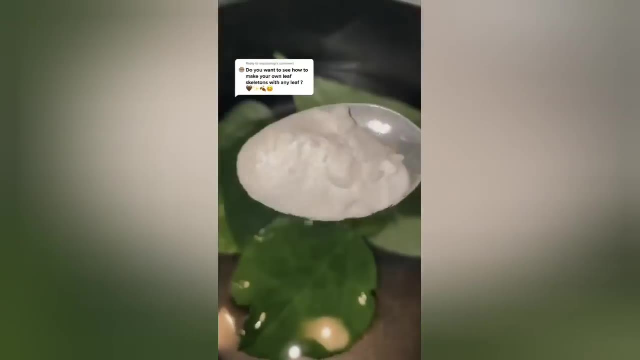 as a rule, it's best to choose leaves with a waxy surface and with a lot of veins on the back. then pop those leaves into a bowl and give them a good wash to remove dirt and mud. add your leaves and water into a boiling pot with one tablespoon of baking soda and let it come to a boil once it has. 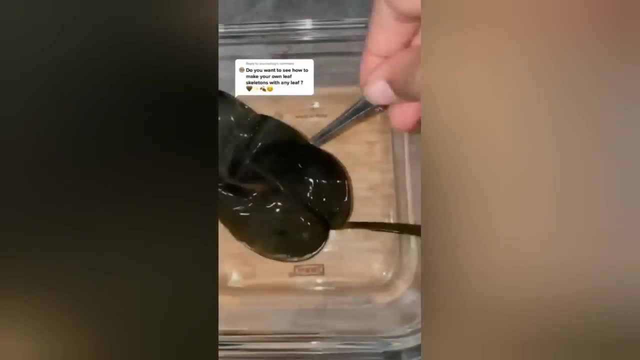 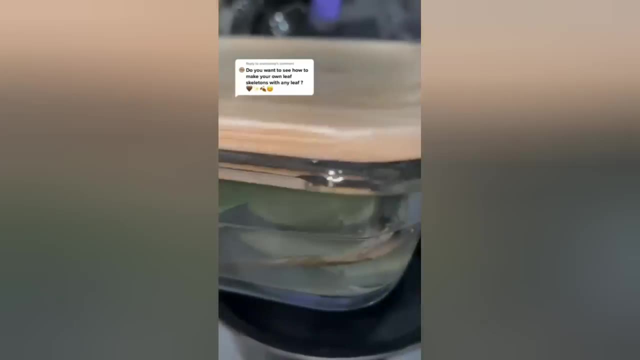 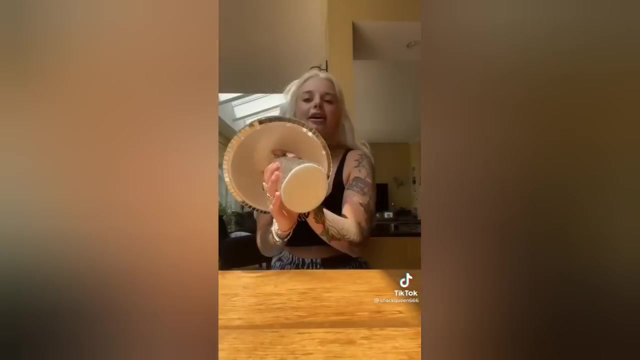 turn off the flame and let it cool down, pop your leaves into an airtight container and cover completely with the same water. then store it for six days to come back for part two. so it's pretty simple. it's just time consuming. i went to the craft store and i got like a foam cone and this foam dome and then i put like a barbecue skewer, like a wooden one to like, hold it up and then glue it all together and then these are mirror tiles off amazon. 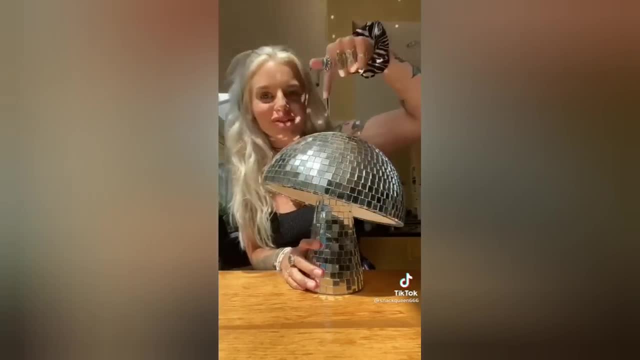 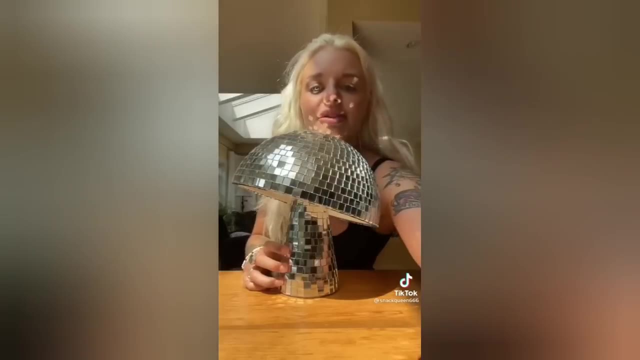 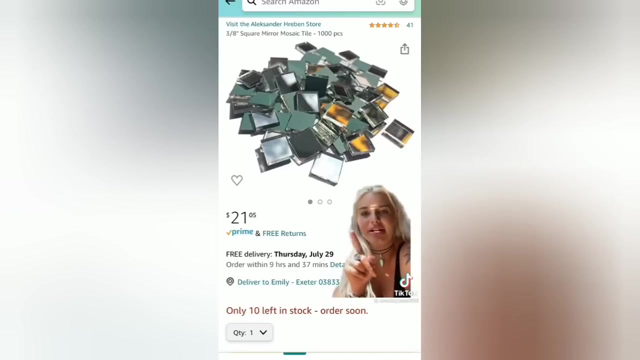 so i ordered this a couple times. it comes with a thousand of these little mirror tiles and i ordered like a million of these, because i ordered just one, and i got a couple big bottles of differentstar- like a million of them. and then I made this mushroom. I also made a wiener, but I 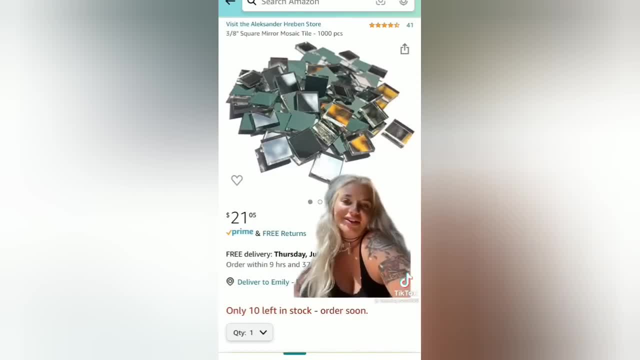 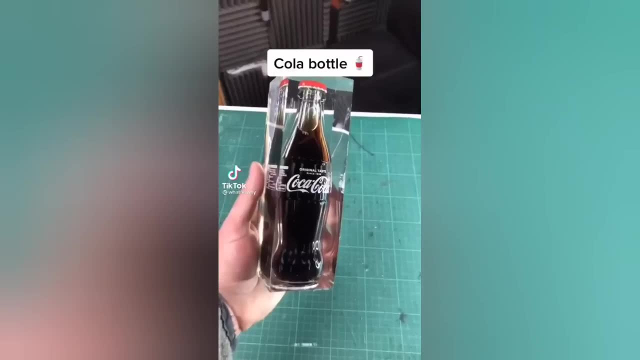 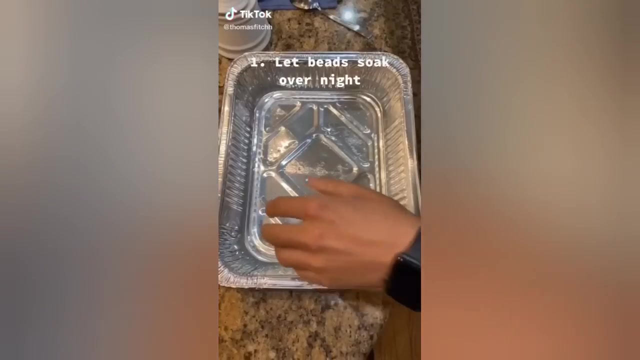 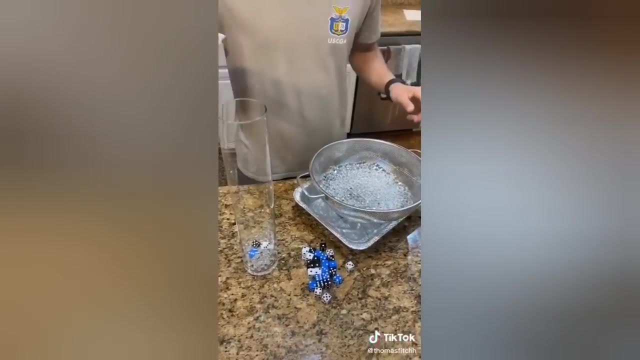 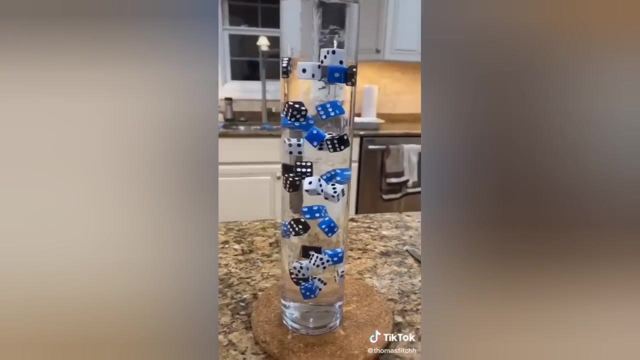 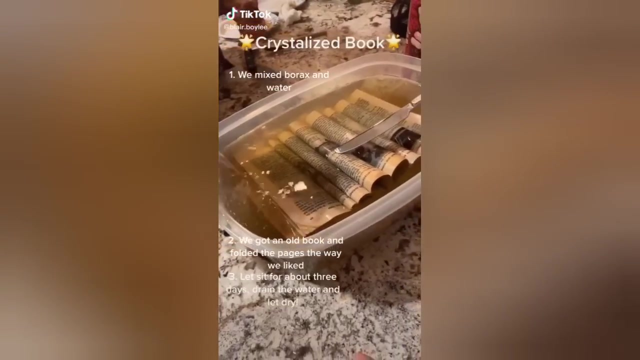 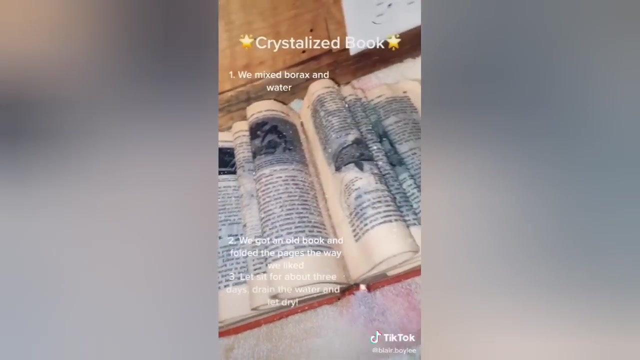 can't show you on here because my videos all get taken down a bit. so craft day. I really like to break Venom on socks when I'm stepping out of sex. I hit it in the morning cause I'm whiskey dicking. Got my, Maybe Let's go. 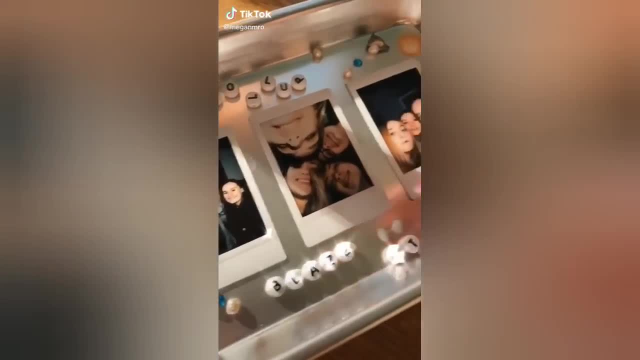 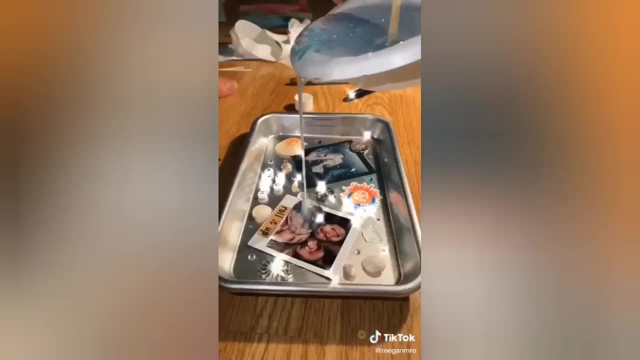 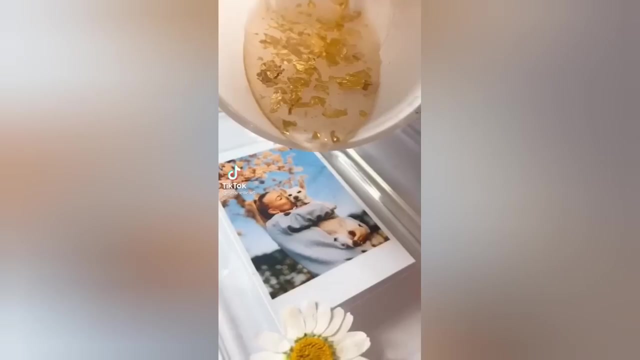 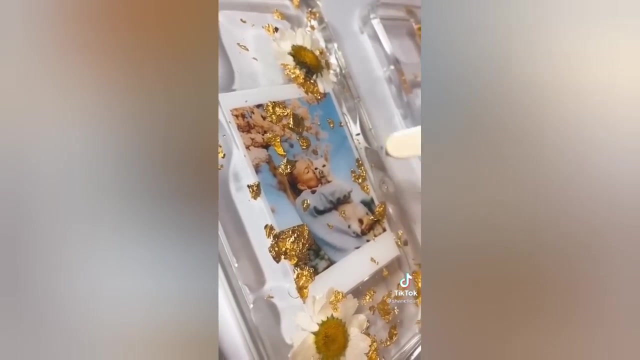 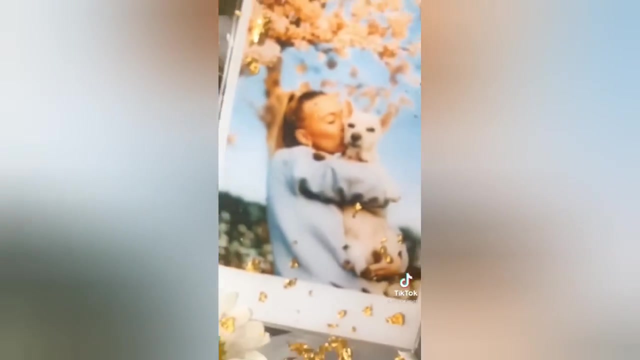 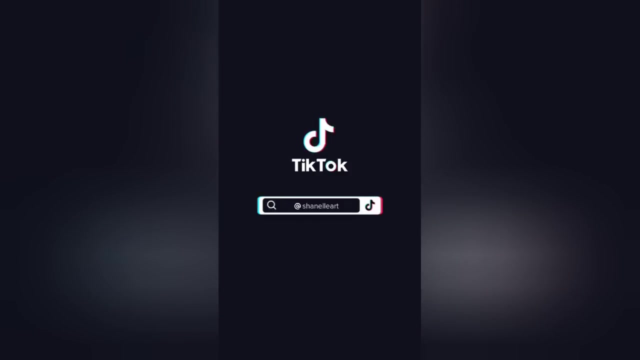 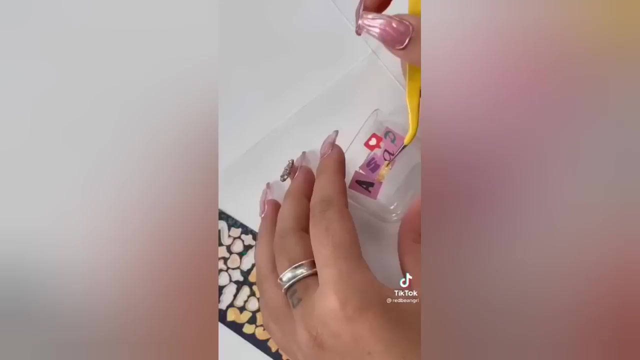 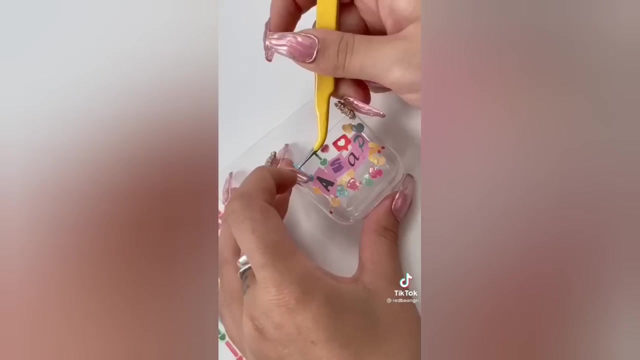 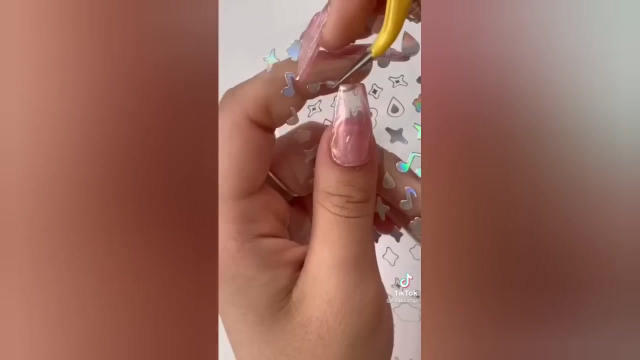 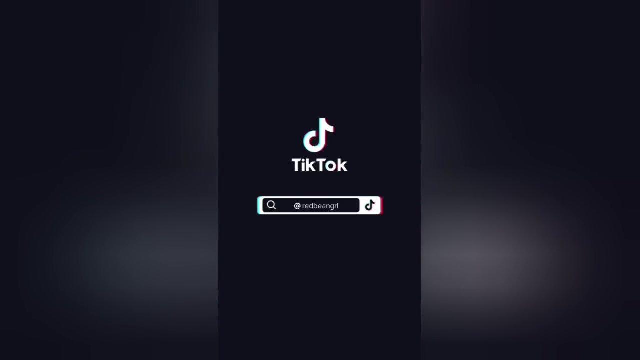 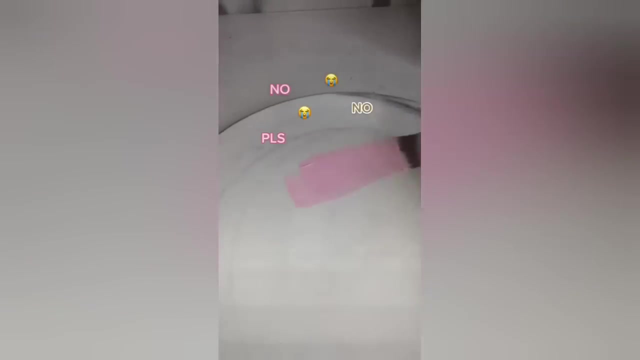 Yeah, Let's go, Let's go, Let's go. Chocolate, No, no, no, no. Please, don't hurt me, Please. Finally, I've been trying to catch you boys all day. Now that I've got you right where I want you, I'd like to buy all your chocolate. 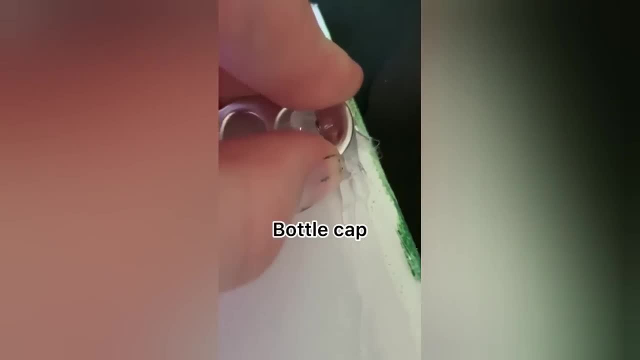 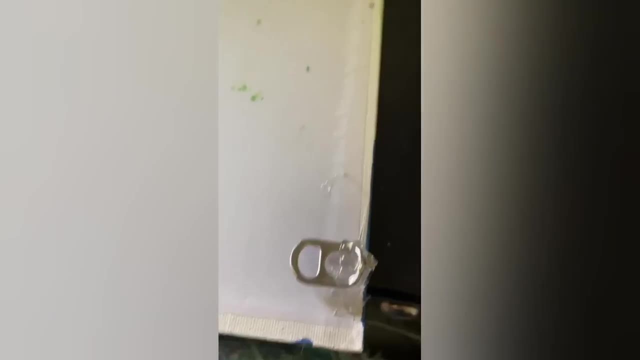 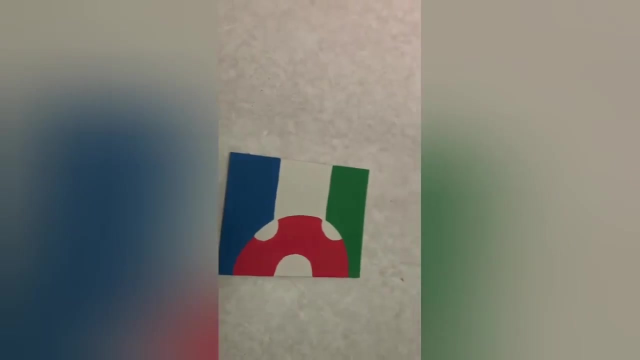 Gets better on the house. I'm not just 18, I'm 16. I would make it, I wouldn't mind. I'm just 20, I'd like to be someone. It's not like it. never traffic, Didn't even make it. You couldssss, Talk to me. 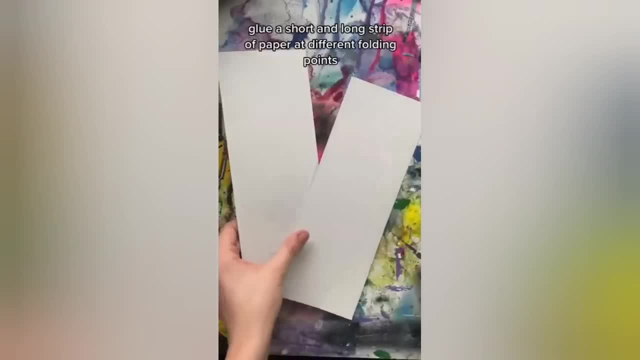 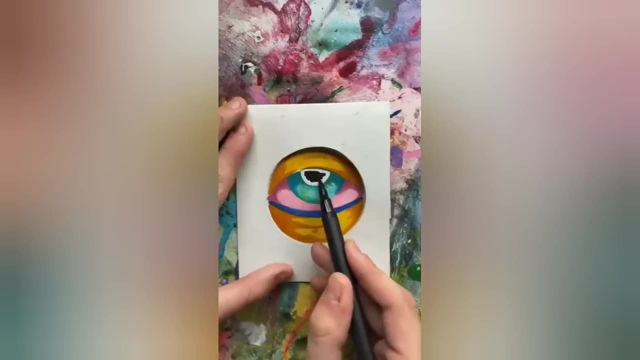 You said you'd only appreciate Slow your fucking with the Beyonce. Huh, Let's go, Thank you. Thanks for watching.